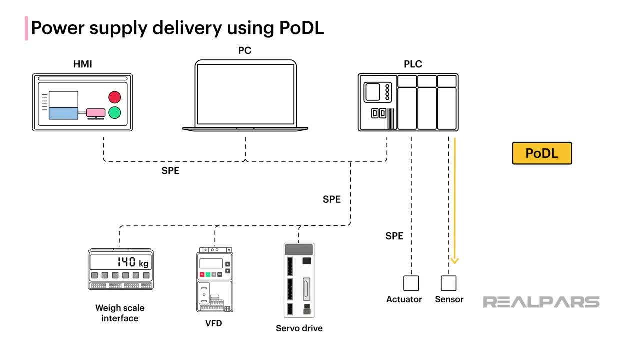 to end devices using what is called PODL or Power Over Data Line. Special cables and connectors allow both power and data to be transmitted over a single cable. Various cable configurations and power capacities are available to deliver up to 16 amps to connected devices. 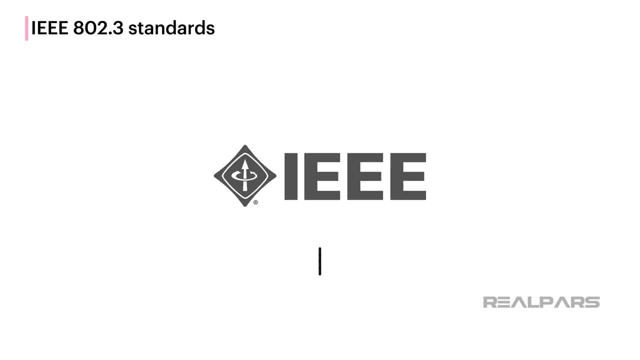 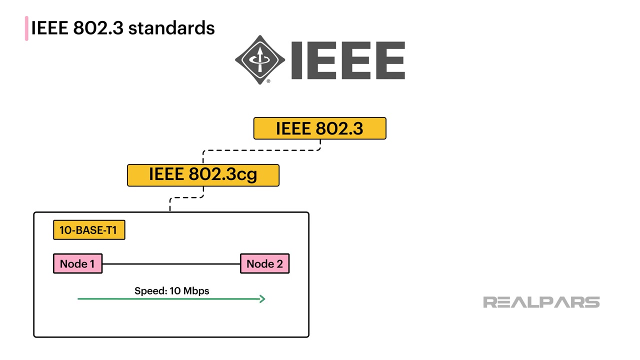 Single Pair Ethernet is represented by a new group of IEEE 802.3 standards. The IEEE 802.3cg standard is most important for the process industries. This standard describes 10 base T1 or 10 megabit per second Ethernet which can be run over a single twisted pair cable up to 100 meters with no loss of signal. 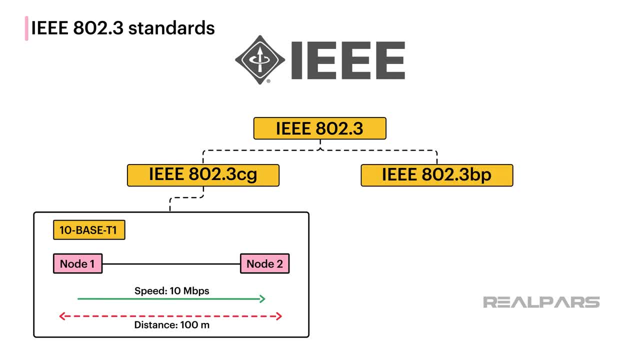 IEEE 802.3bp is most important for the process industries. IEEE 802.3cg standard is most important for the process industries. IEEE 802.3cg standard is most important for the process industries. It is the standard with a higher data rate of 1 gigabit per second. 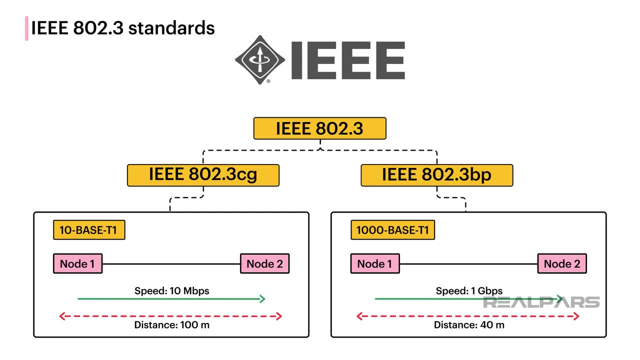 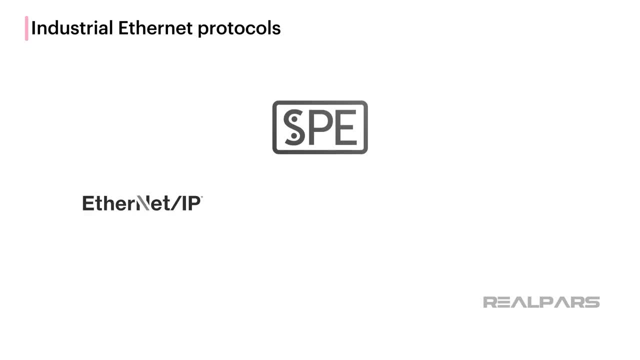 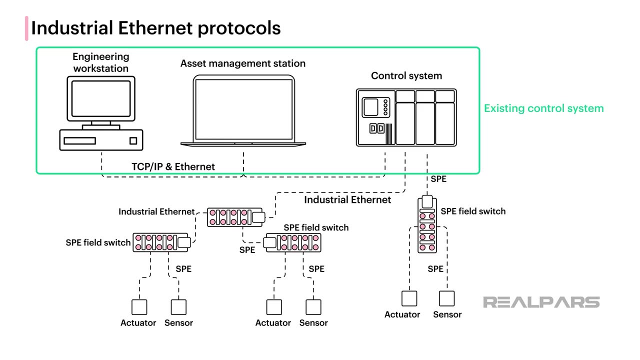 but with shorter lengths of up to 40 meters allowed. Single Pair Ethernet communicates across the common industrial Ethernet protocols available today, such as Ethernet-IP, PROFINET and EtherCAT. This allows existing control devices, such as PLCs, which operate on these industrial Ethernet protocols. 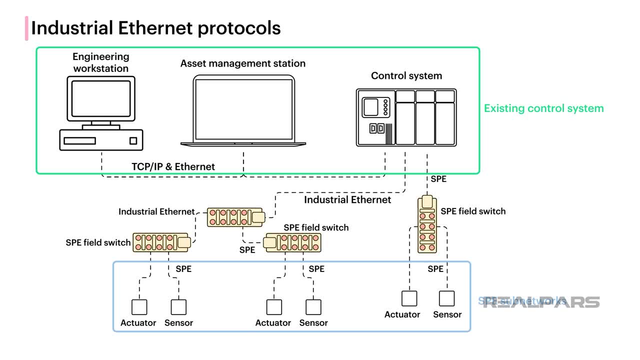 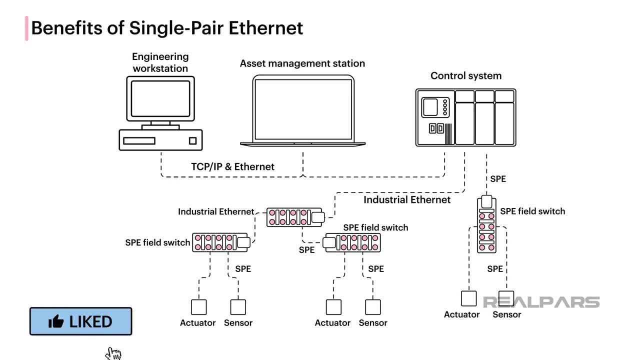 to interface to Single Pair Ethernet. This allows existing control devices, such as Ethernet-IP, PROFINET and EtherCAT to interface to Single Pair Ethernet sub-networks via the use of SPE field switches. The use of SPE field switches and Ethernet-connected devices. 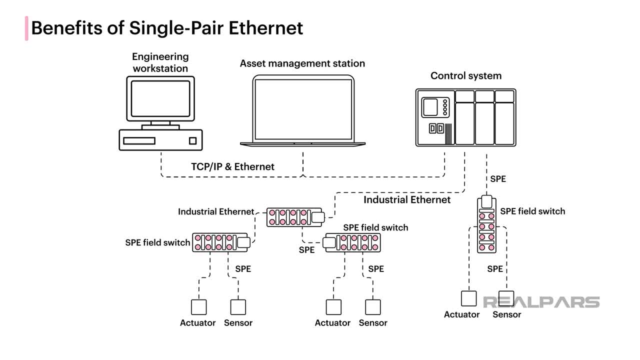 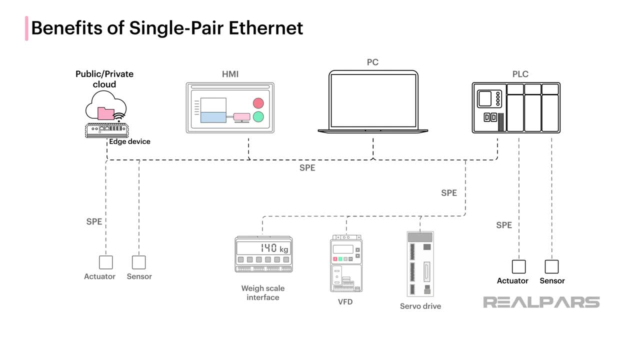 means IP communication can be brought down to the lowest automation level, offering full transparency from sensors and actuators all the way up to the cloud. Other benefits of Single Pair Ethernet include reduced wiring costs, reduced node costs, reduced power consumption and data communications via a single pair of wires. 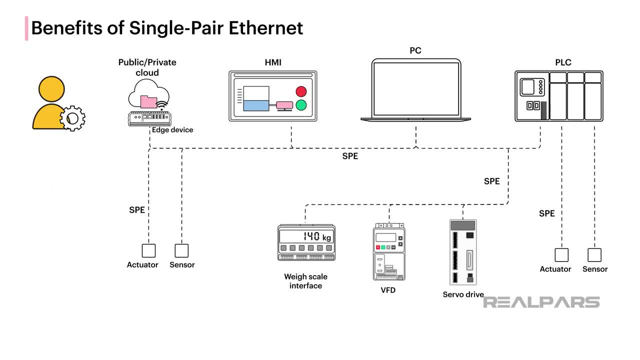 IP technologies are very familiar to engineers, technicians and operators alike. Being able to use a single network type for all plant-level communication will flatten learning curves and eliminate the need to learn the nuances of many types of networks. Single Pair Ethernet using Power over Data line is not the same as Power over Ethernet. 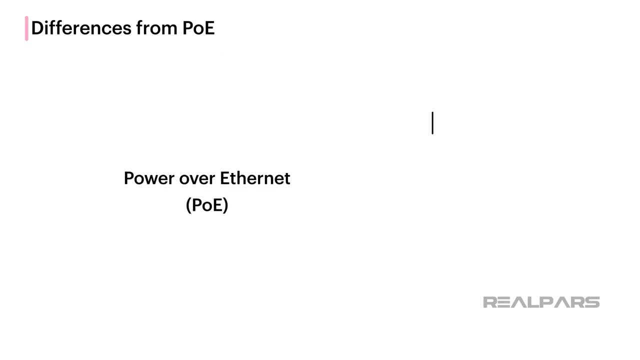 often referred to as Power over Ethernet, often referred to as PoE. Power over Ethernet is described by IEEE standards 802.3af, 802.3at and 802.3bt. PoE requires a special network switch with one device connected to each port using a Cat5 cable. 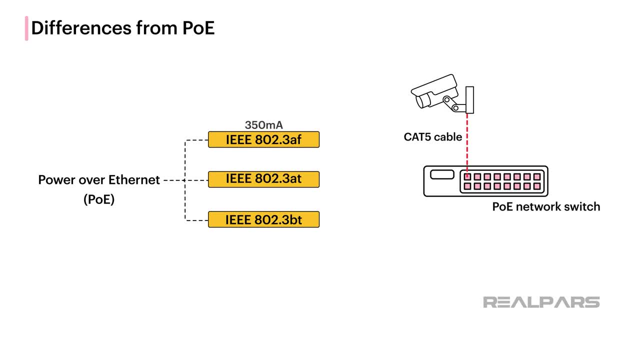 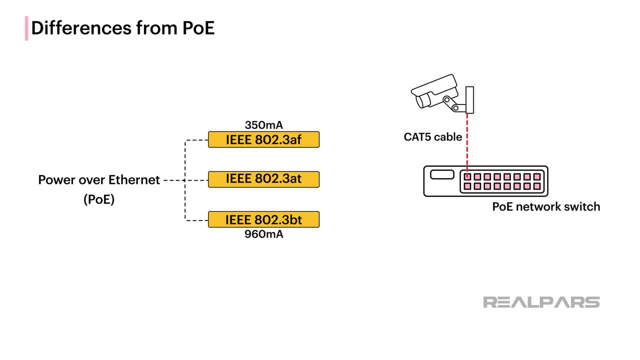 For IEEE 802.3bt power is limited to 360 mA. PoE has been useful for connection of devices such as wireless access points, voice-over internet phones and monitoring cameras. The physical network limitations of Power over Ethernet limits its usefulness for the integration of plant-level sensors or field devices. 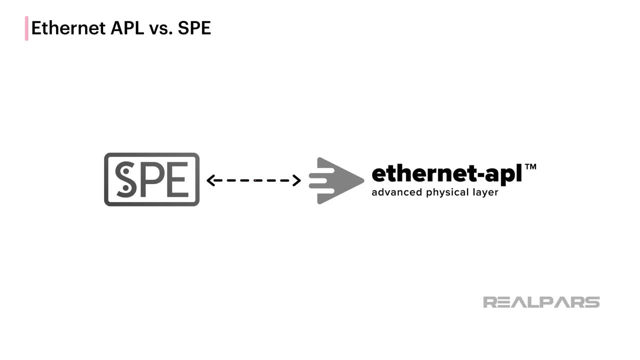 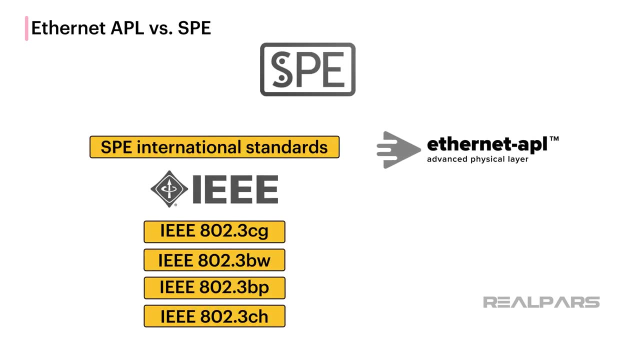 Single Pair Ethernet and Ethernet APL are not interchangeable terms. As mentioned before, there are two types of Ethernet and there are several IEEE standards that define the different versions of Single Pair Ethernet. Ethernet APL for Advanced Physical Layer is a specific version of Single Pair Ethernet. 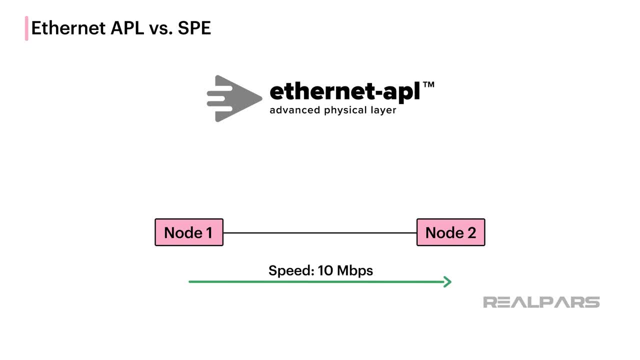 Ethernet APL operates at 10 megabits per second, defined as 10 base T1L, where the designation of L indicates a long distance, in this case 1000 meters. Being able to extend Ethernet to these distances will allow Ethernet. 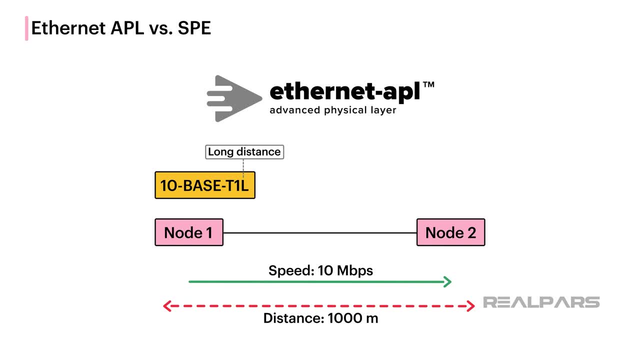 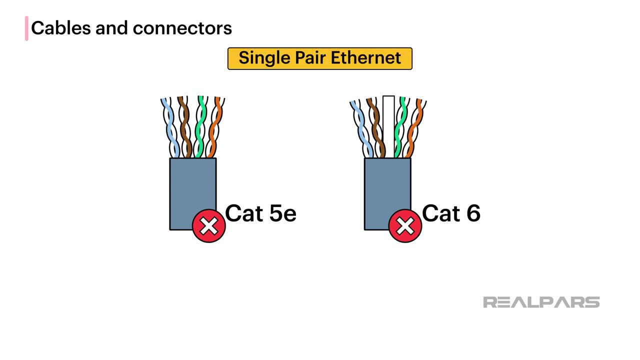 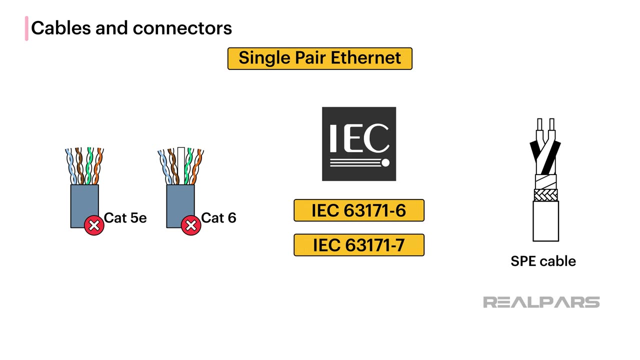 to be employed where it has not been able to previously in manufacturing plants. Conventional Cat5e and Cat6 cables cannot be used to connect Single Pair Ethernet devices Cables as defined by standards IEC 63171-6 and IEC 63171-7. 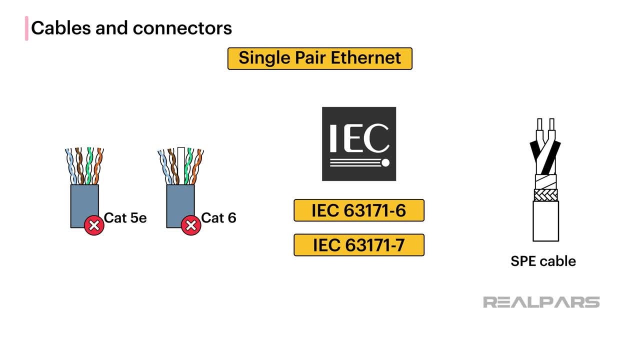 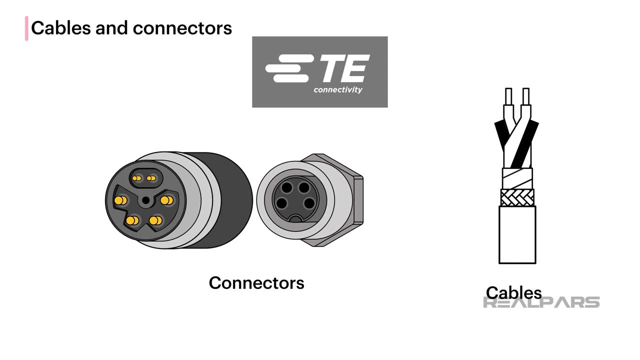 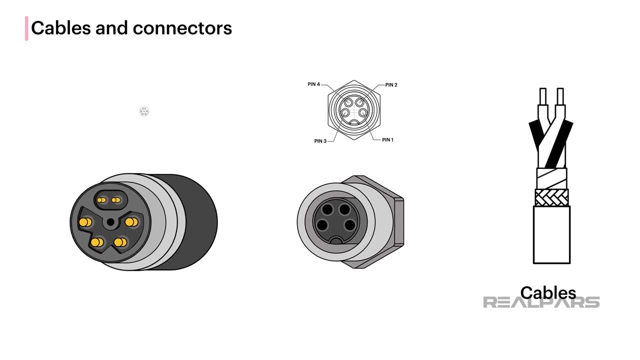 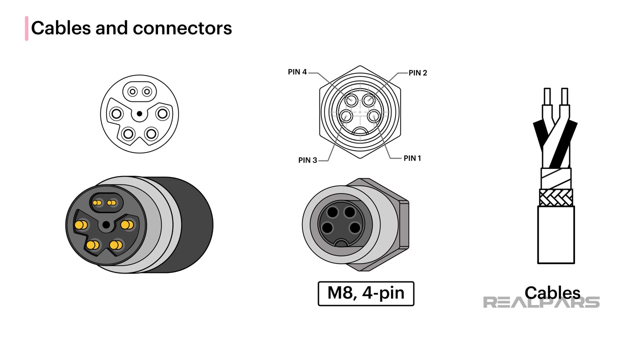 have been developed for SPE to ensure interconnectivity between SPE devices. Automation suppliers, such as TE Connectivity, are engineering and manufacturing these new cable and connector configurations to support SPE networks. Power and data are delivered to the devices over a single cable using 4-pin M8 connectors or 6-pin M12 connectors. 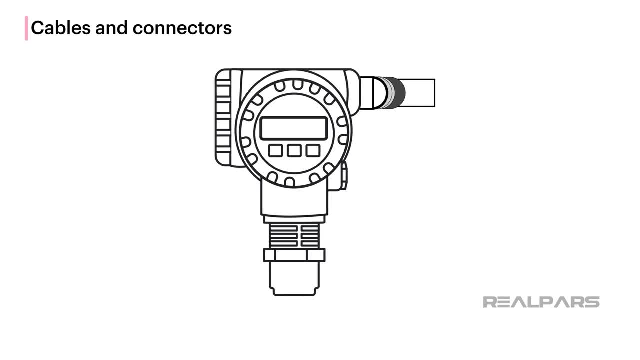 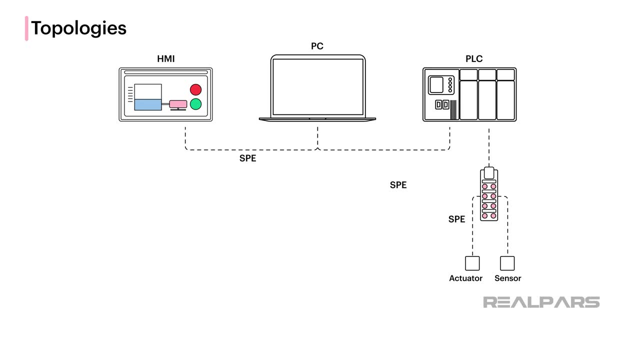 These quick connect cables eliminate the need for cable glands, removing the sensor housing and making screw terminations. Single Pair Ethernet networks are designed to support SPE networks, and these networks can be constructed to connect devices and sensors in a number of different topologies, including Point-to-Point. 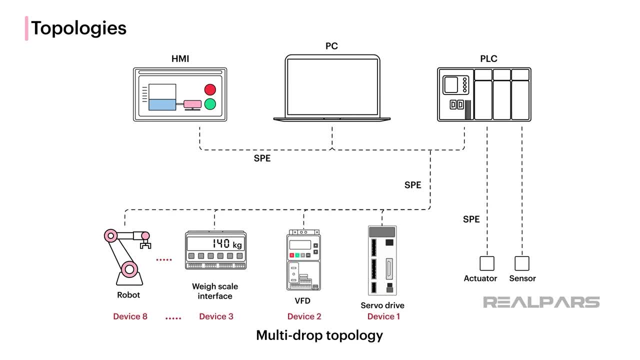 and Multi-Drop for connecting up to eight separate devices. A Multi-Drop topology requires a terminating resistor at each end of the segment, the same as Profibus, Dp and Foundation Fieldbus field networks. Hybrid Multi-Drop Connection technology will enable single-band networks to connect to one network. 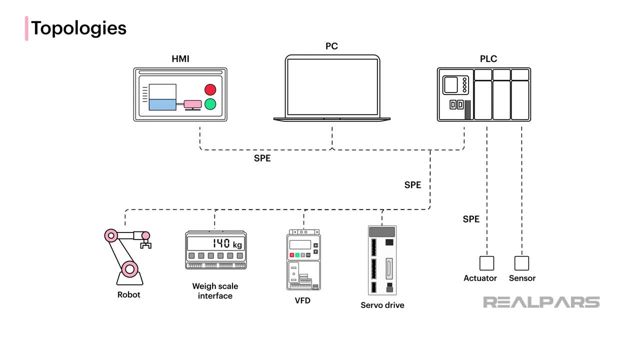 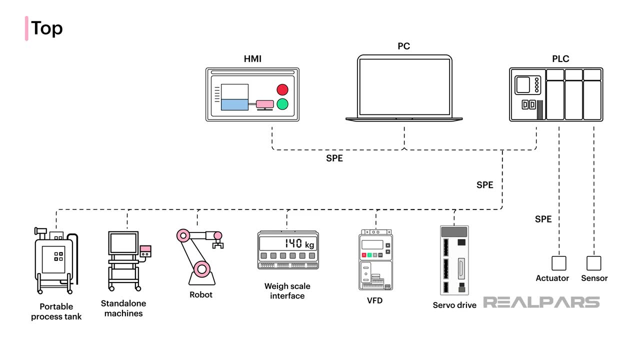 along with a multidrop connection module which will connect the entire network to one network. A Multi-Drop technology will enable single-band connection to connect to one network, single-point network connections to stand-alone machines, robots and portable process tanks, just as a few examples. 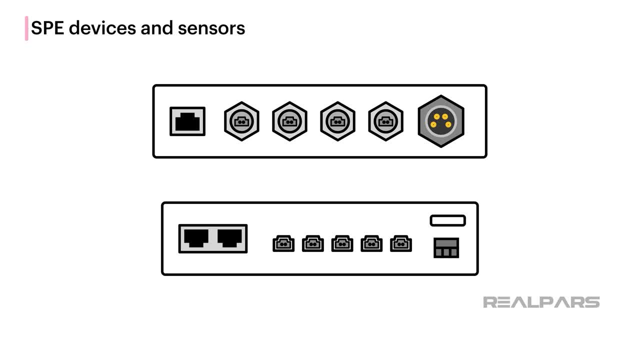 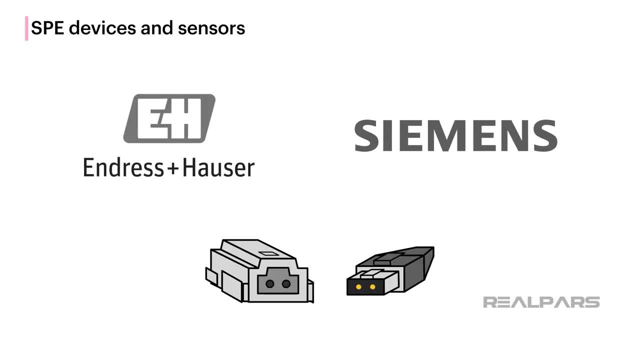 While several manufacturers have SPE field network switches available, SPE-enabled sensors and devices are not yet being marketed. Major automation suppliers such as Indris and Hauser and Siemens have developed SPE interfaces for many of their sensors and many are currently in the testing stages prior to release. 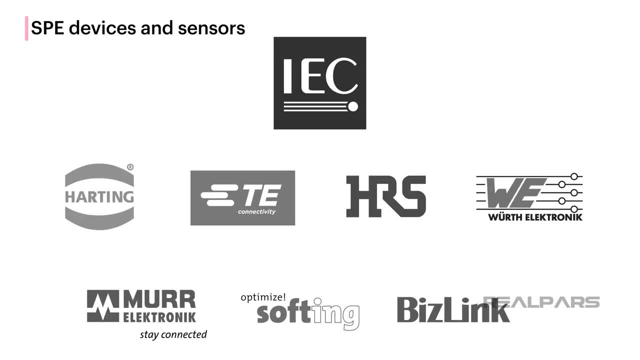 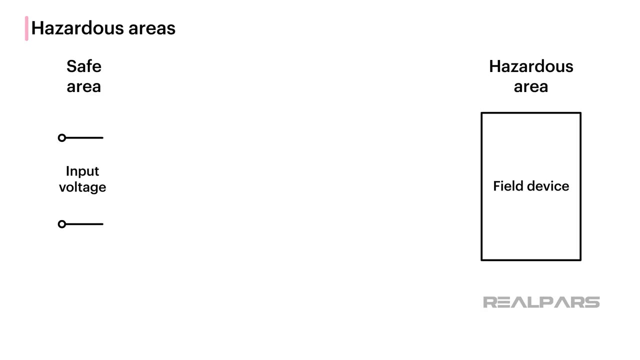 The single-pair Ethernet industrial partner network is composed of a number of very reputable automation suppliers and growing These partner networks will help drive the release of SPE products to the marketplace over the next several years. Electrically classified areas pose additional burdens on automation engineers. 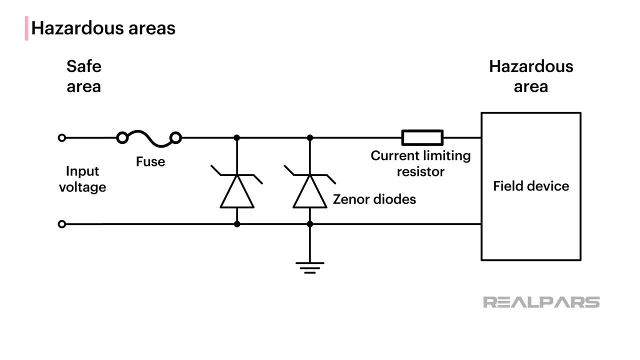 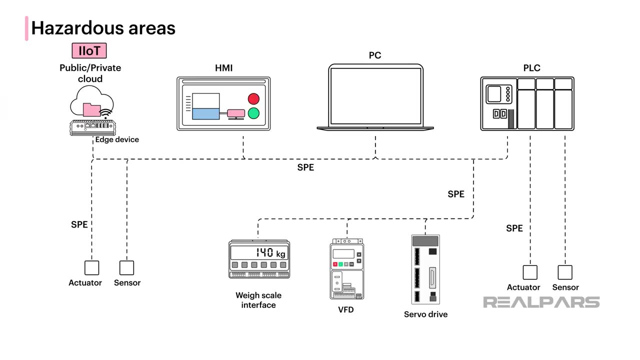 in the design of systems that are safe for use in hazardous areas. Single-Pair Ethernet- Industrial Partner Networks Ethernet, along with advances in intrinsically safe barrier technology for communication networks, provides an opportunity to extend Ethernet to these plant-level areas. Therefore, a single-network strategy can be employed from the field to the cloud. 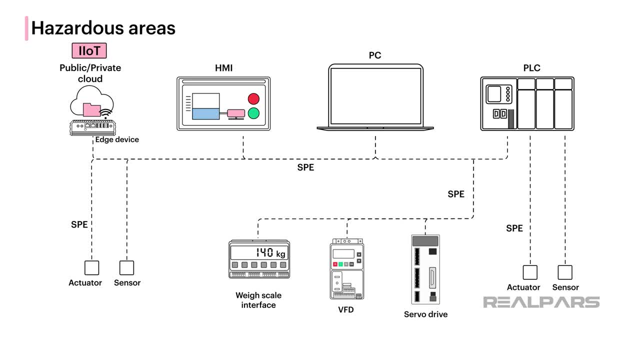 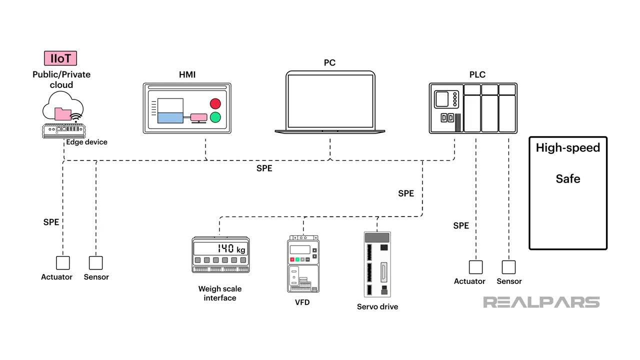 by changing only the physical installation details to match the process environment. Single-pair Ethernet holds the promise of providing high-speed, safe, secure and robust communication from the plant floor to the cloud using IEEE 802.3 Ethernet. The benefits are numerous, from lower cost, simplified installation.